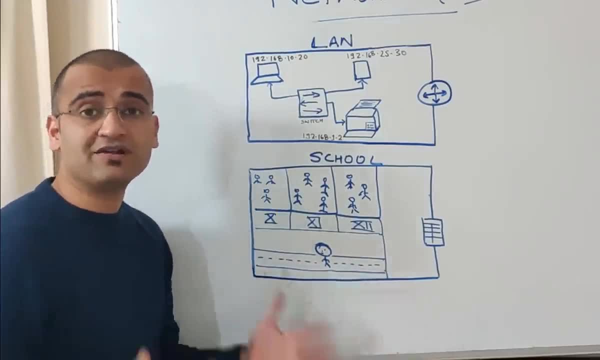 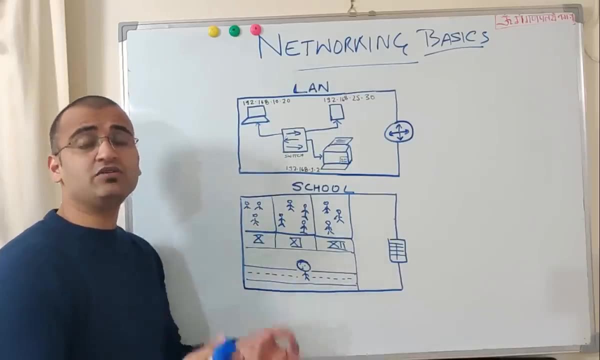 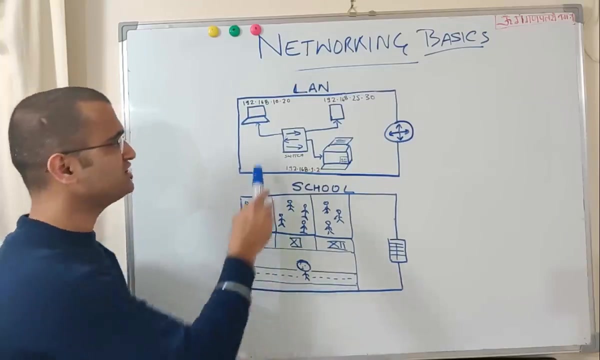 can consider these students as different devices like a laptop a printer or a mobile every student in every class has a unique role number with which he or she is identified that particular role number can be identified as an ip address moving on the next concept is a switch what is a switch so switch is a device which sits within your local area network and helps you talk to 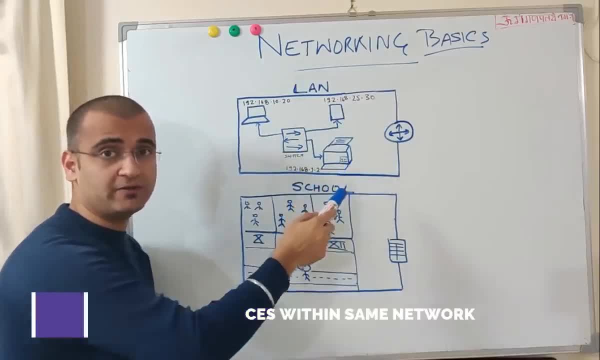 which kind of device are they that are identified by these device as a local area network so the site will be identified in your local area network which in some cases are the devices which won't place various devices within your local area network range. 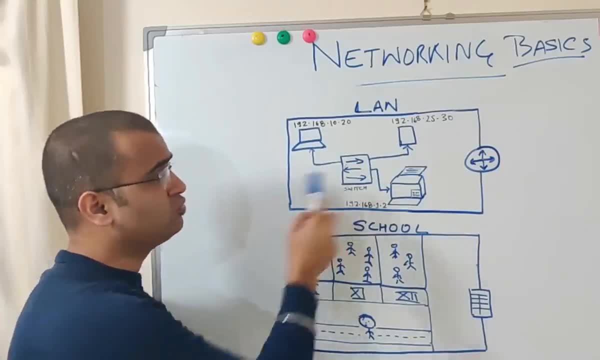 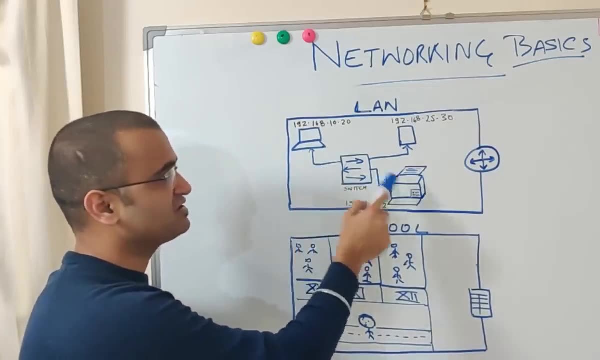 Suppose if you want to print a copy of your file from a printer, then you can simply send your request and switch will identify that, okay, this request needs to go to this particular IP address. 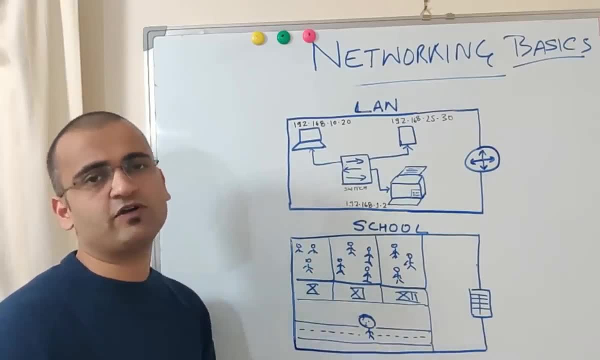 So switch specifically works within a closed range of a local area network. So in a school, if suppose a class 10th student wants to go and meet a student of class 12th, 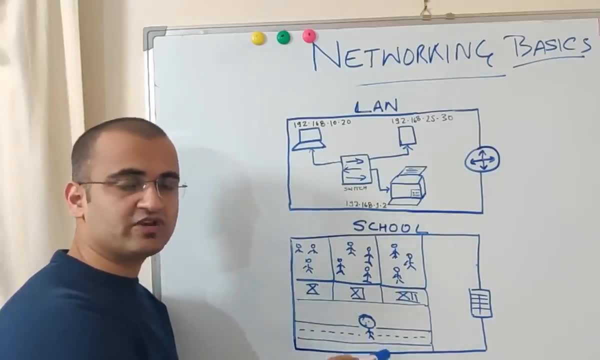 he has to first go to this peon and he has to take permission and tell him that I want to talk to this specific student and this is his roll number. 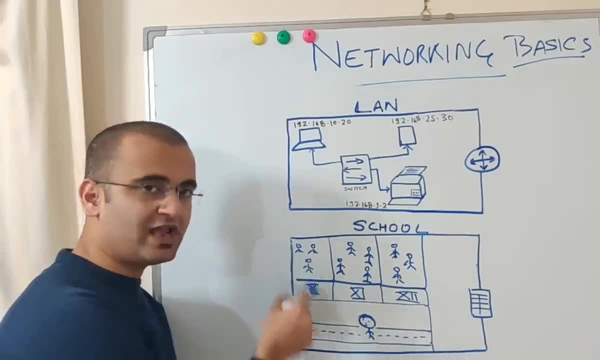 And based on that, this peon will pass on the message or allow this particular student to go and meet the student of class 12th. 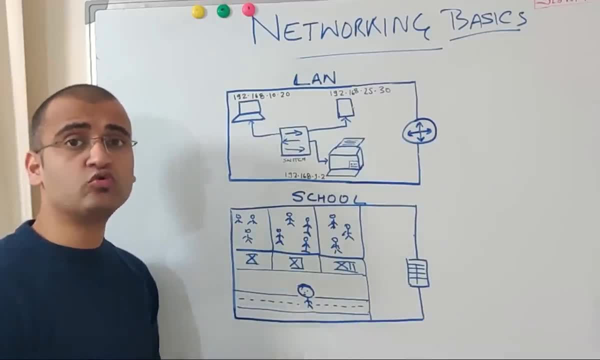 But what if student of this particular school wants to go and meet a student of a school next to this particular school, but that school is outside the boundaries of this particular school. 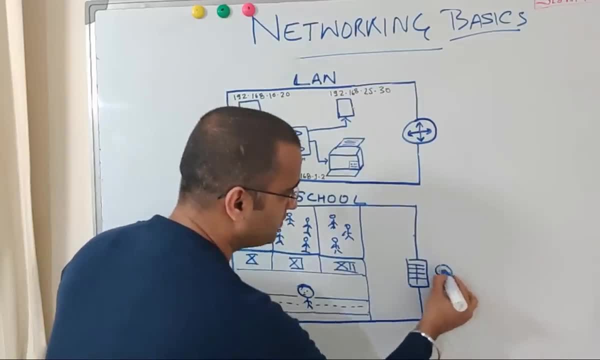 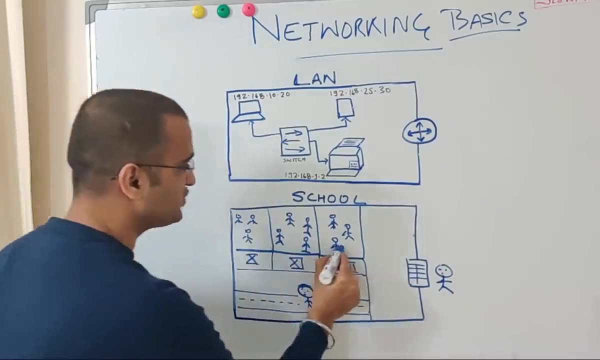 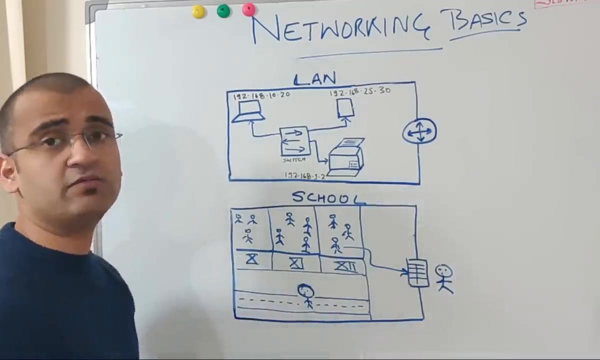 In that case, this student has to go and meet the main security guard here, which is there at the main gate, main security gate. And he has to ask permission of this particular security guard and only then he can go and meet someone outside the school boundaries. So this is security guard is nothing but a router. Okay. 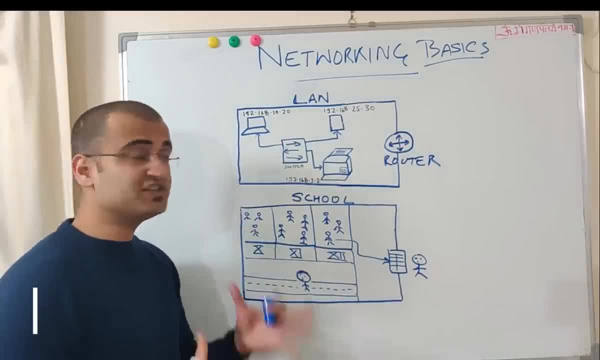 So a router is a network device which sits between our local area network and the outside network, which is a wide area network. 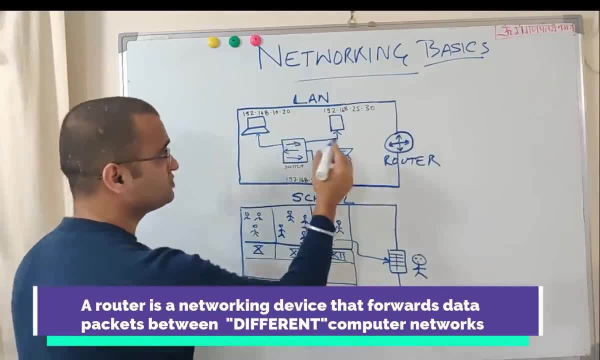 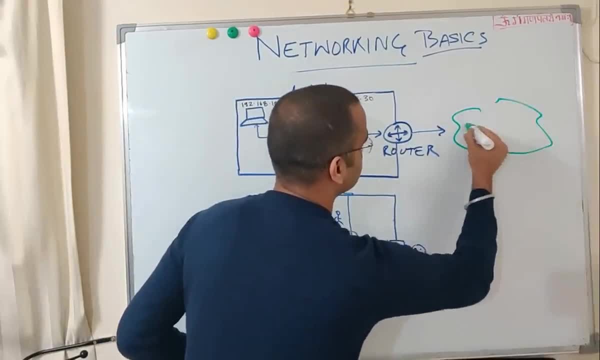 So suppose our mobile wants to connect to the internet, then this mobile will send requests to the router and then this router will connect to the outside internet. 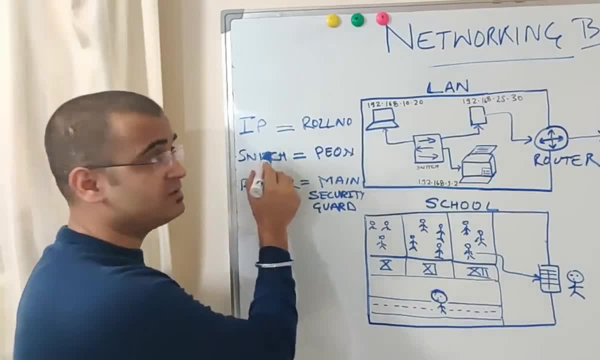 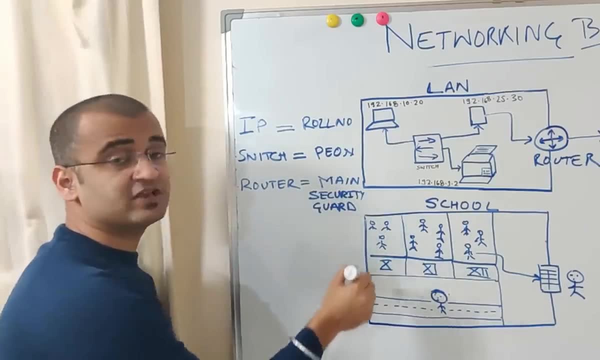 So to draw some analogies, IP of any machine can be a roll number of any student. A switch can be this peon and a router can be the main security guard, which allows you to go outside the, uh, outside your school or go outside the network. 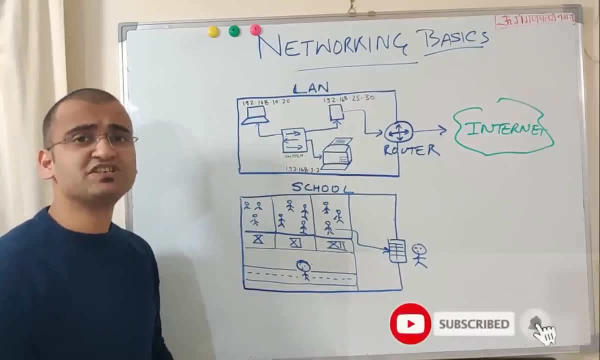 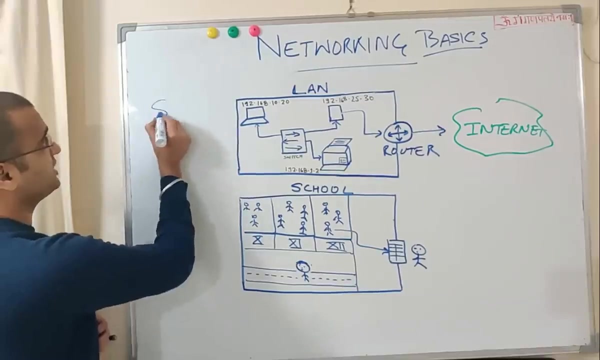 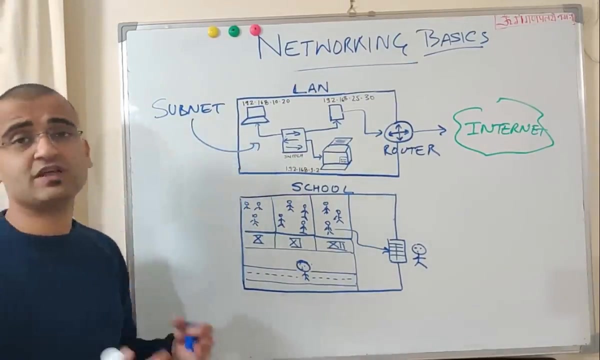 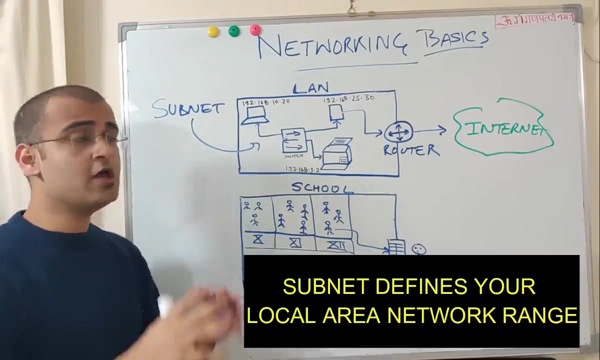 But the question arises how a machine would know whether a machine sits within the local area network or it is sitting somewhere outside the main local network. How a machine can understand that that can be done through yet another concept, which will, which is called a subnet. So subnet is called as a subnetwork, which sits within the local area network and it is not an IP address. It might look like an IP address, but it is not. It is a set of flags, which defines the overall range of a local area network. I'll tell you how. 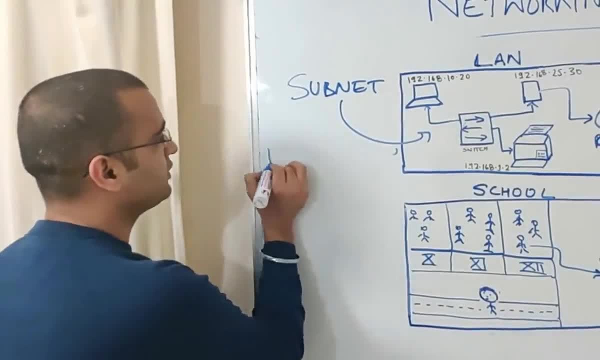 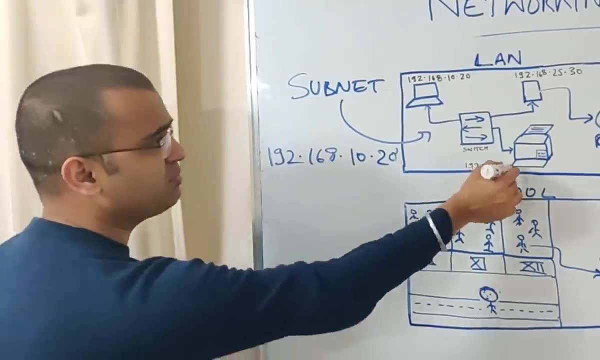 So suppose the IP address of this particular laptop is 192.168.10.20 and the IP address of this printer is. 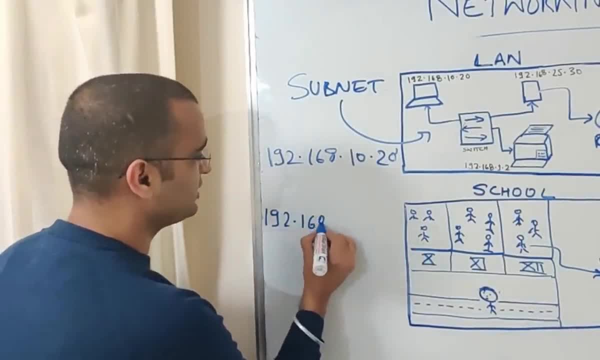 192.168.1.2 between these two sits the subnet. 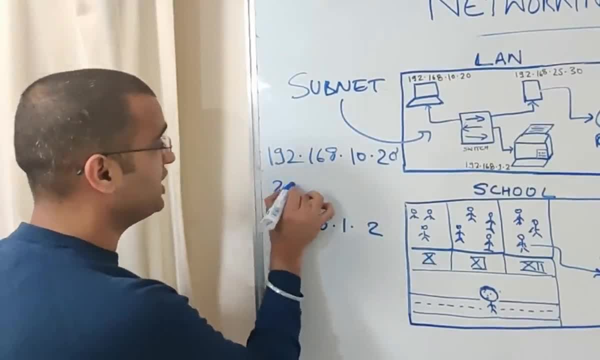 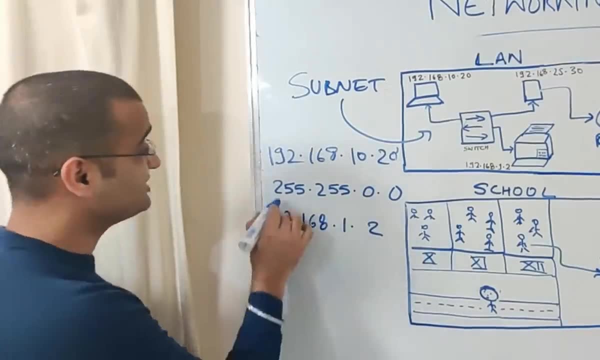 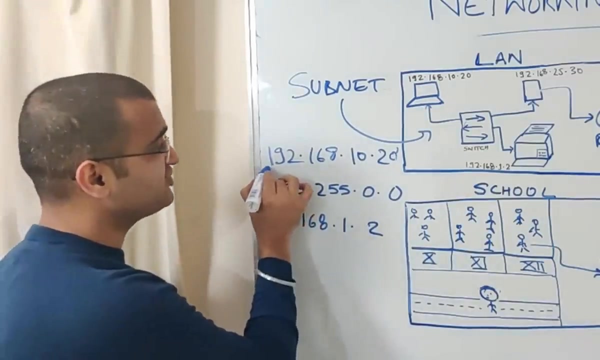 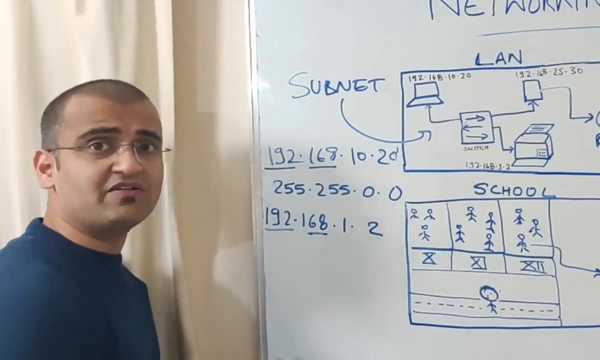 So subnet for this particular local area network could be 255.255.0.0. What does this mean? These are the flags. These two 255 flags denotes that this particular local area network has a fixed range of 192.168. So any device which falls within this particular IP address range would potentially be the device in the local area network. 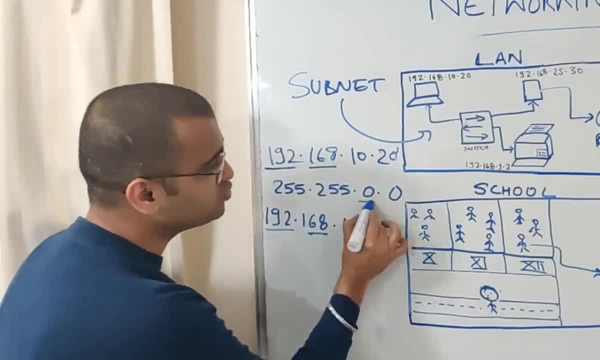 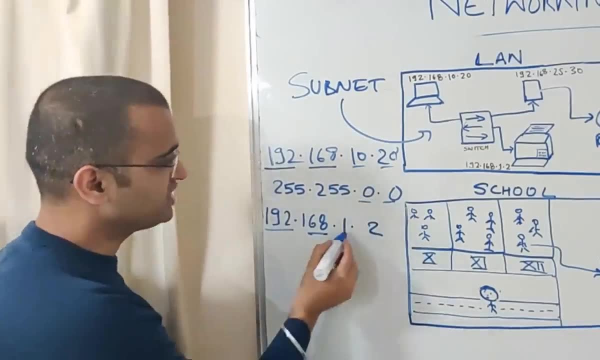 If suppose this particular IP address matches, then these two zeros denotes the free range. There can be any number sitting in these last two categories because these are zeros. So it can be 1.2 or it can be the mobile 192.168.25.30. So subnet decides your local area network. Okay. 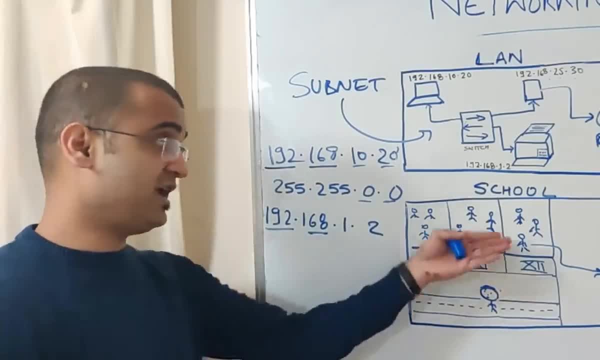 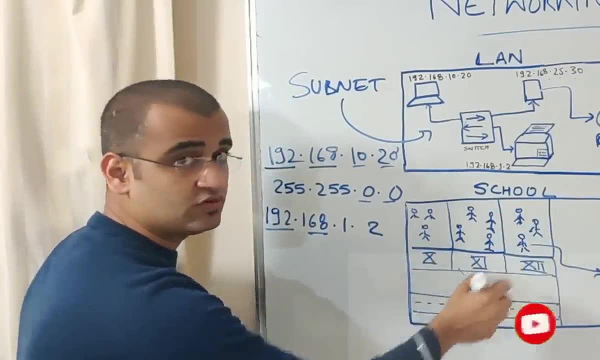 So if you want to correlate with a school example, then the roll number of one student and the roll number of another student can identify, we can identify whether they belong to the same school. 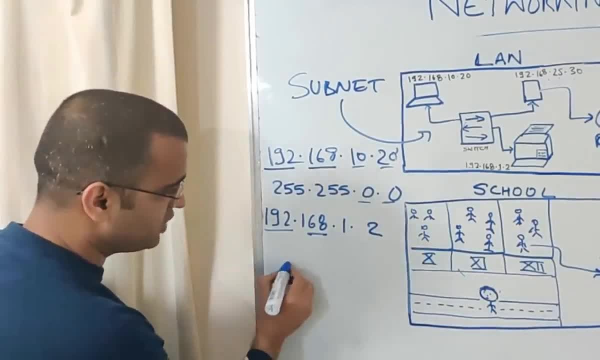 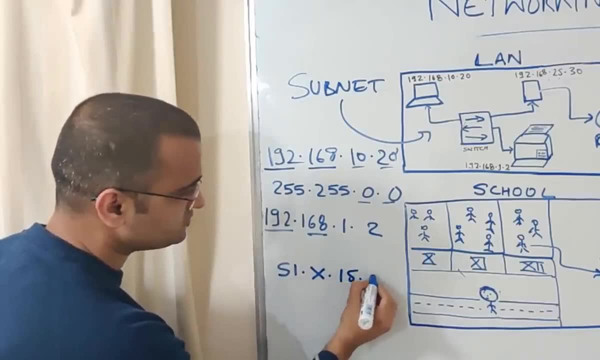 So a student of class 10th can have a roll number like S1, which denote the school 10.15.5. And the roll number of the 12th student could be S1.15.5. Okay. 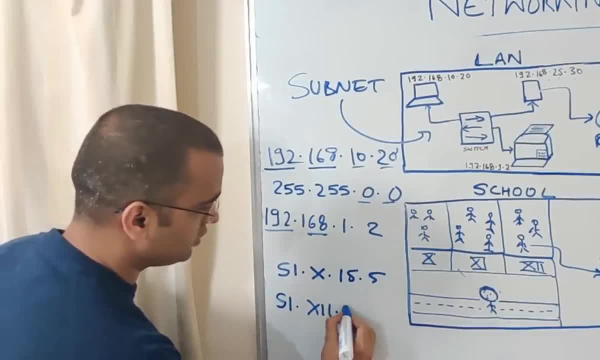 So to use this, let's take the maximum number of 2 persons who are not sunny. Let's say 1.24 is your total number of the student. 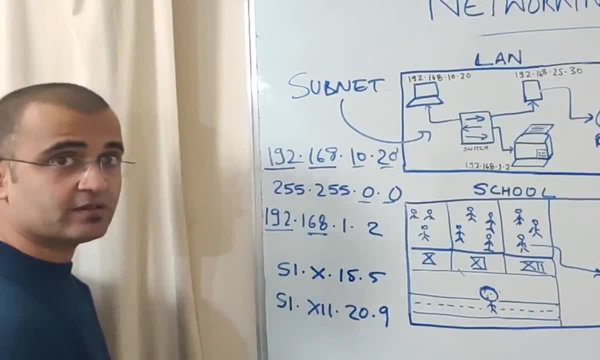 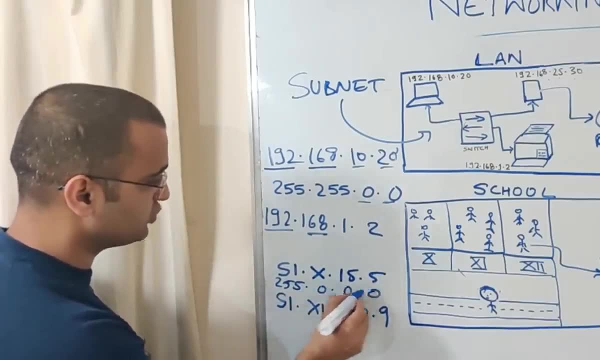 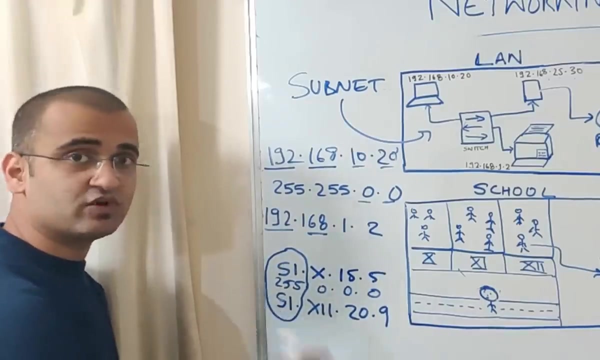 Now, you might observe the of four students in your class. Boys and girls, let's talk with them. 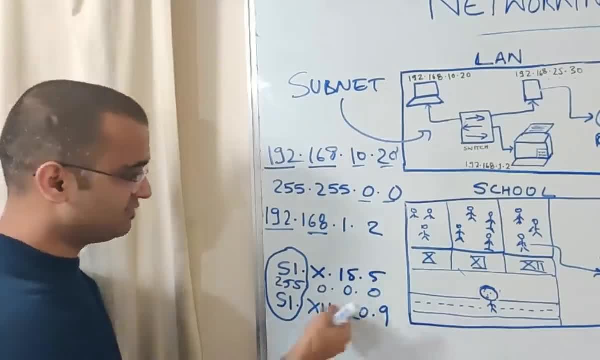 Okay. So what should we do? Can you see it? None. Okay? None. So you can check your 7.25.f please. one. 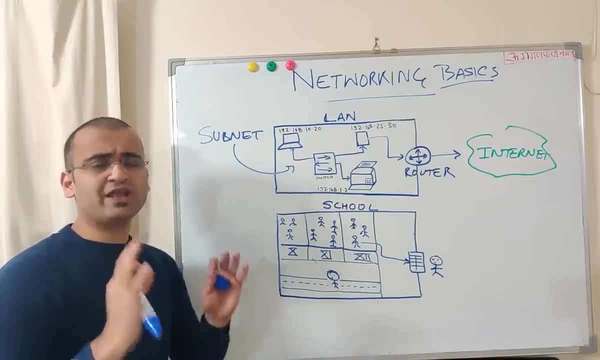 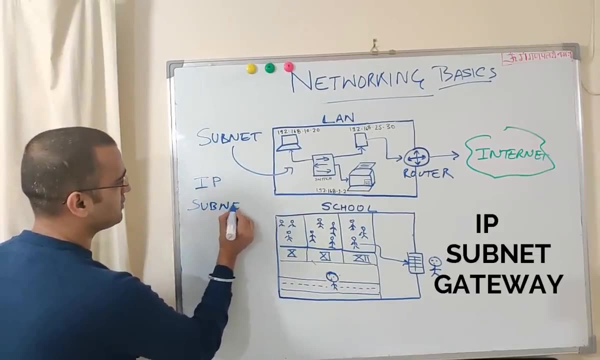 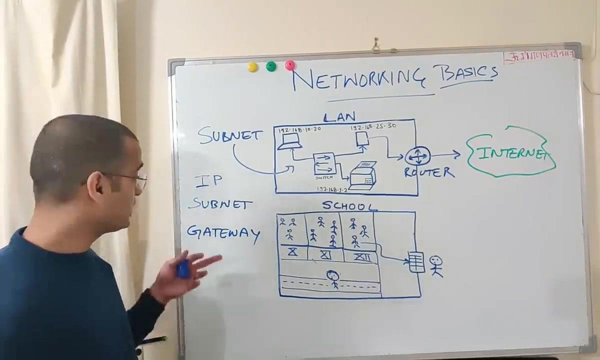 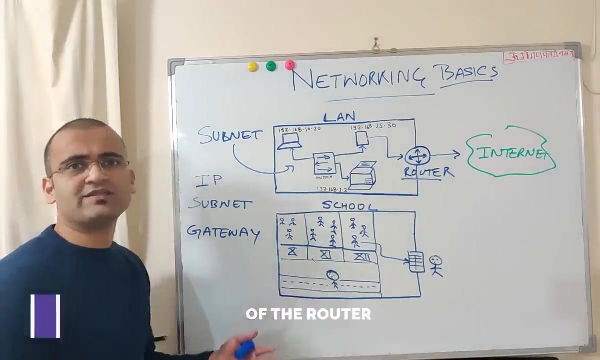 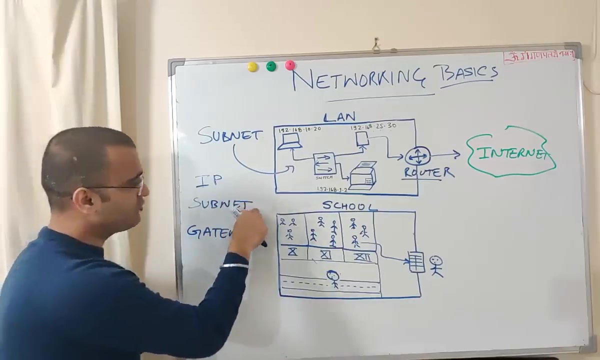 network so to summarize any network device potentially needs three things IP subnet and gateway now you will now you will wonder what is this gateway gateway is nothing but the IP address of this router so router and gateway are one and the same thing the IP address of the router is actually called as the network gateway so this IP address along with this subnet and this gateway can pretty much talk to any other network network device within the LAN or outside the LAN so hope I am clear on this concept now we will move on to the leg 2 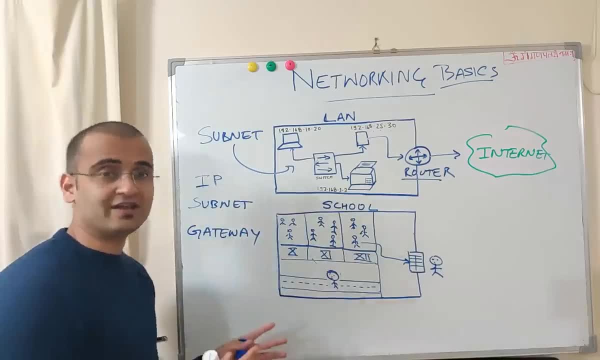 of this video wherein we will understand some concepts on the wider area network so let's start so hope we are clear on leg 1 which covered the LAN concepts now 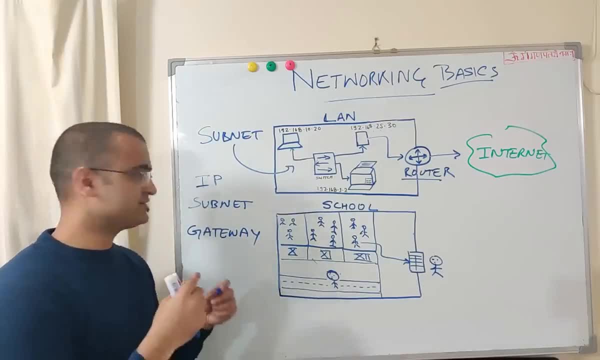 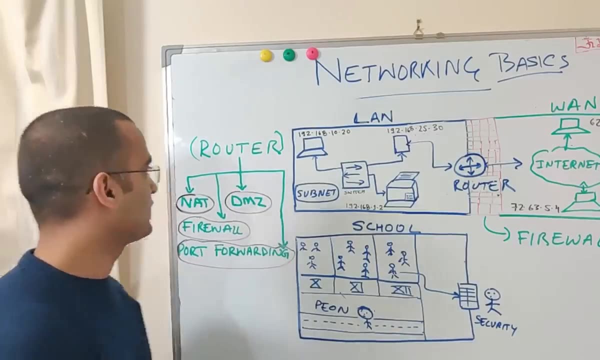 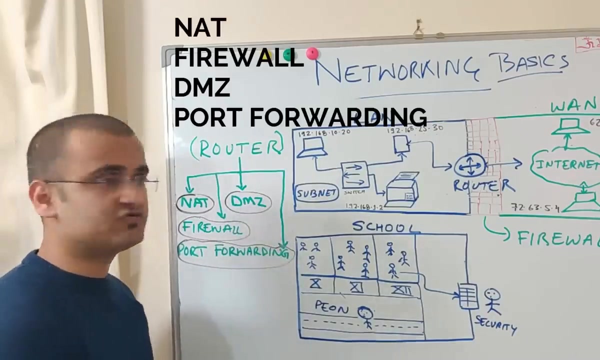 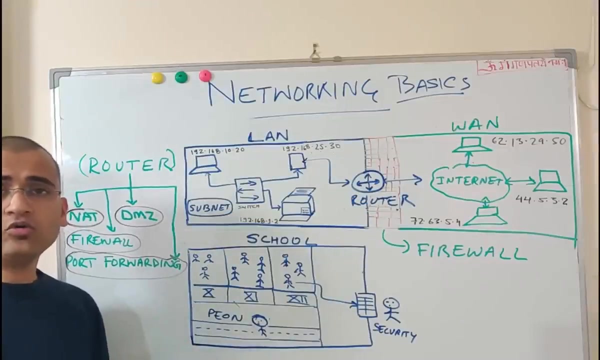 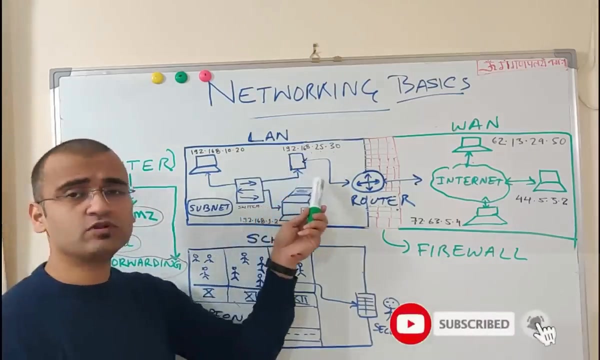 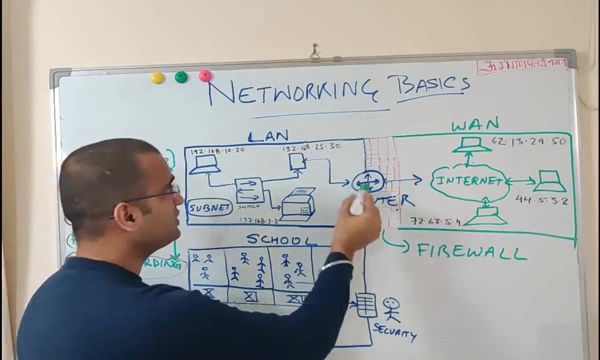 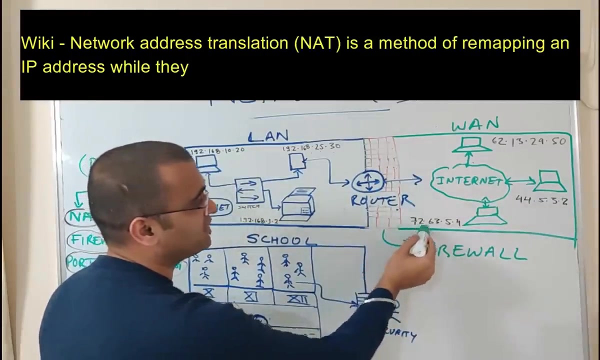 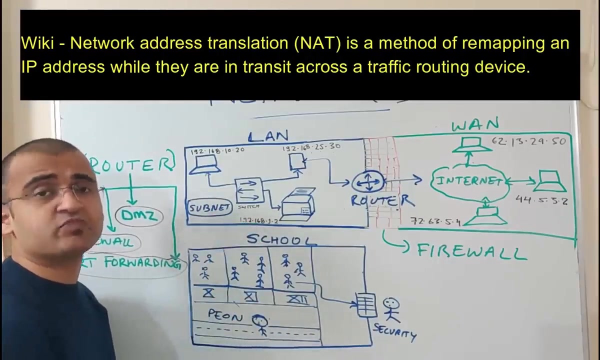 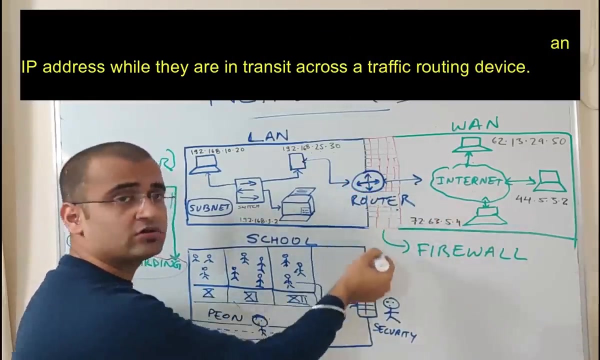 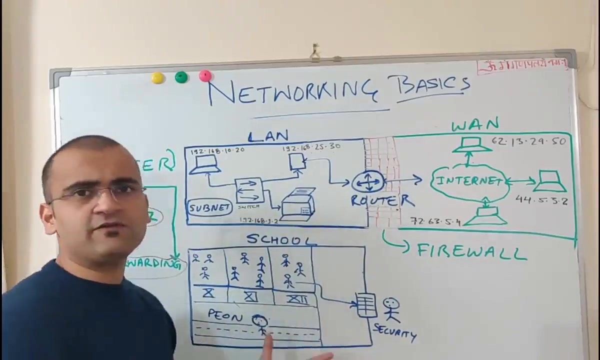 concepts or related to router and wider area network so let's start so router has basically four core functionalities which it has to deliver as a gateway device first is NAT which is network address translation second is DMZ which is demilitarized zone third is firewall and fourth is port forwarding these are all interrelated we'll understand how so we now know that router is the gateway through which a local area device can talk to a device outside the network but but what is network address translation the name pretty much describes it so whatever request comes from the local area network device the IP address of this particular device is not exposed to the internet router changes this network device address to a different address which then goes on to the outside network as you can see the IP addresses of these network devices outside the local area network are different these are all starts from 72.63 where in our subnet starts from 192.168 that's why whenever any device goes outside to talk to another device via the router or the gateway then that particular network address gets translated so a normal flow 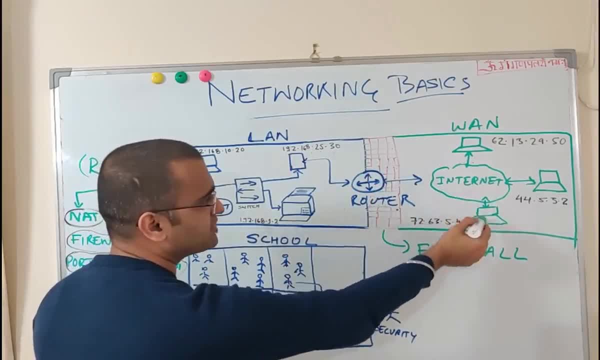 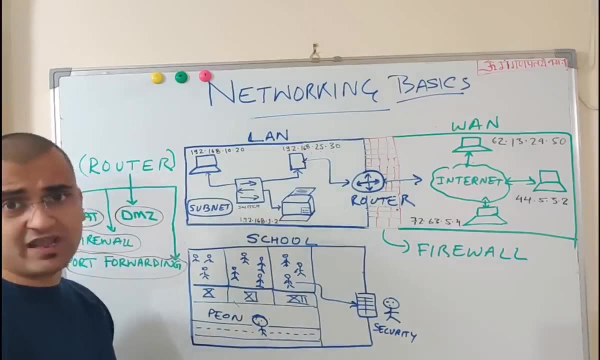 would be a device would go to the router router will request that particular data from a device in the wide area network and then that would be sent back to the the device but what if a device which is completely isolated somewhere in the network wants to talk 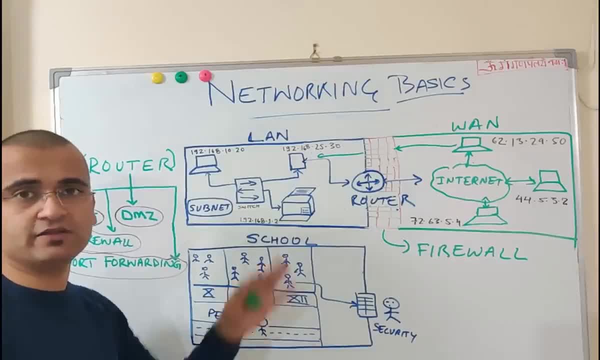 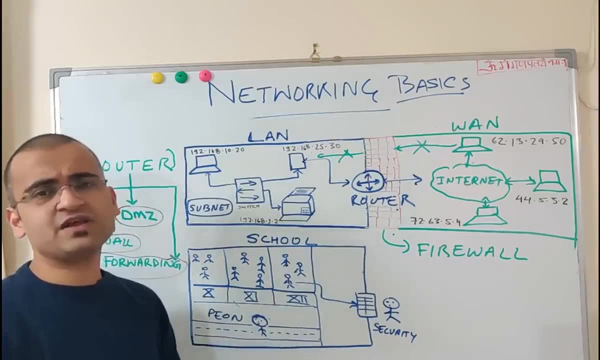 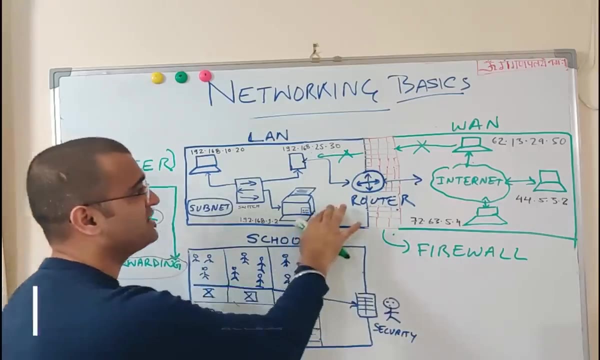 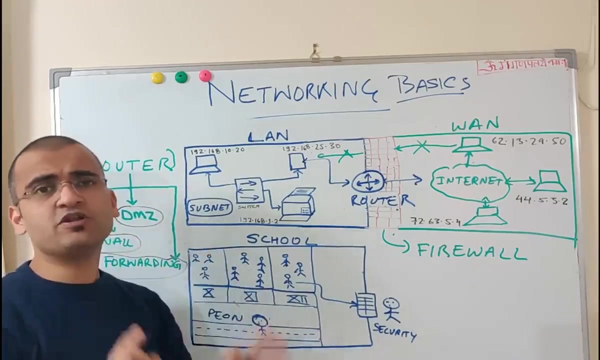 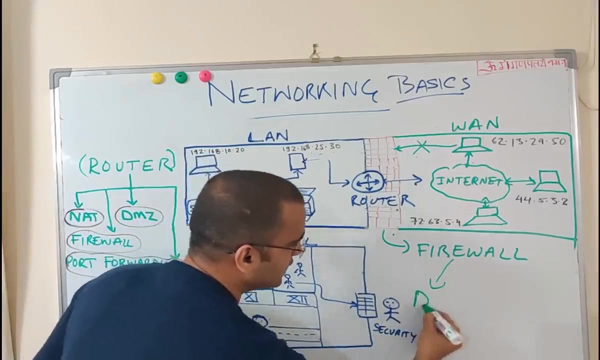 directly to this particular device in the local area network that cannot happen that's a security risk that's why the firewall comes into picture firewall is nothing but a set of passive rules which are defined to enable the set standards of communication between the internal and the external network through this firewall only a specific set of communications can happen and these sort of ad hoc requests cannot that's why if you want to allow any sort of communication through this firewall what are the options you have so you have two options you can either 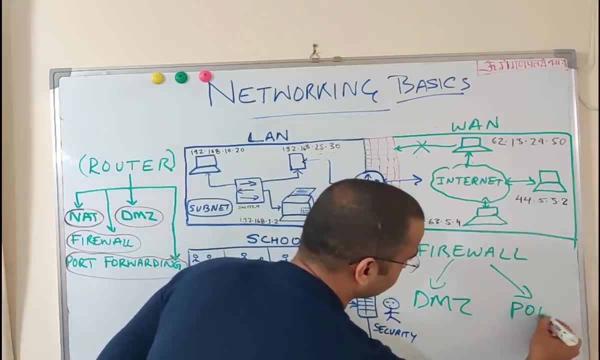 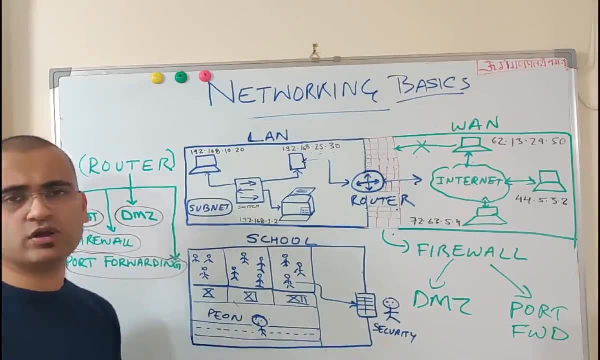 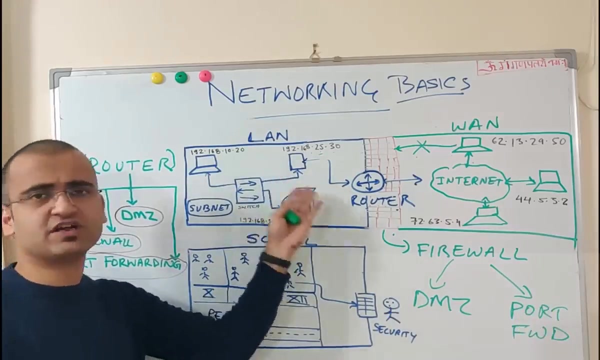 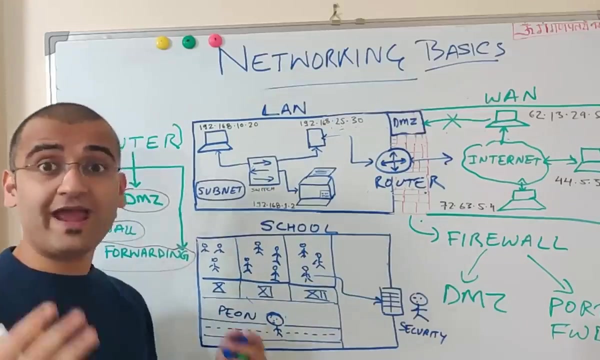 configure a dmz or a port forwarding we'll understand these two concepts quickly what is a dmz dmz is demilitarized zone demilitarized zone is a zone created within the local area network wherein it has it is specified to the router that whenever any ad hoc external network connection wants to try to establish a connection with the local area network you simply pass on that connection to the dmz so if any request comes from an ad hoc device it is it comes to the router and router 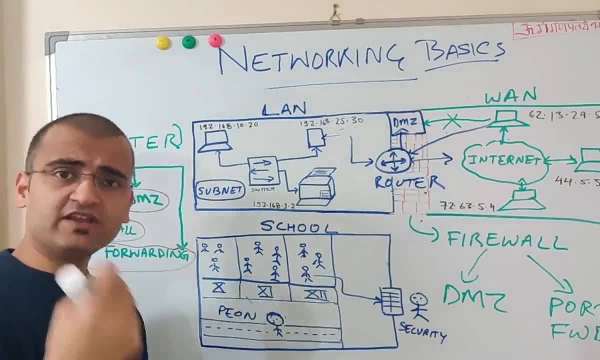 simply send it to this demilitarized zone and if there is any device which is sitting here in the demilitarized zone that device can directly talk to the device outside the firewall 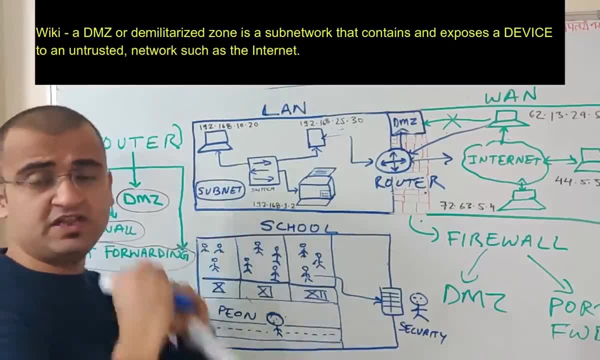 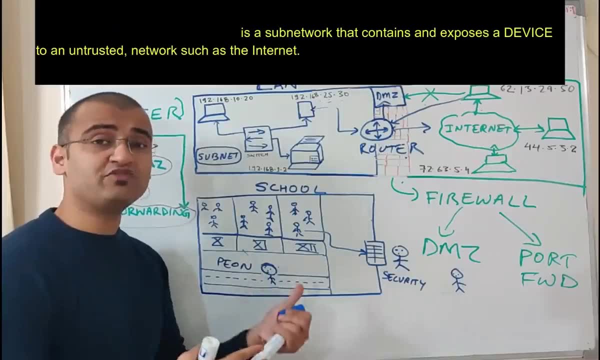 but then the security of this particular dmz and the device sitting with within this dmz is the responsibility of dmz or the device to correlate dmz with a school example 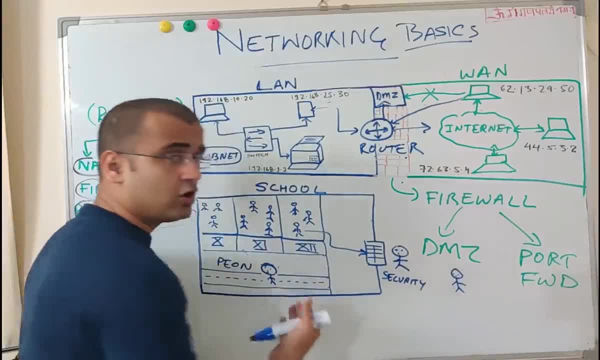 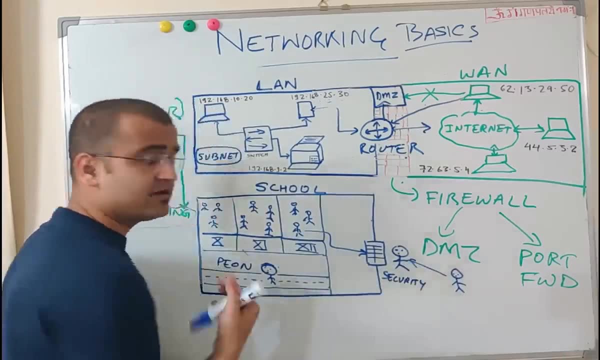 we can correlate it like this suppose a parent or a guest wants to meet certain student in the school he will come to this particular security guard and request for that meeting 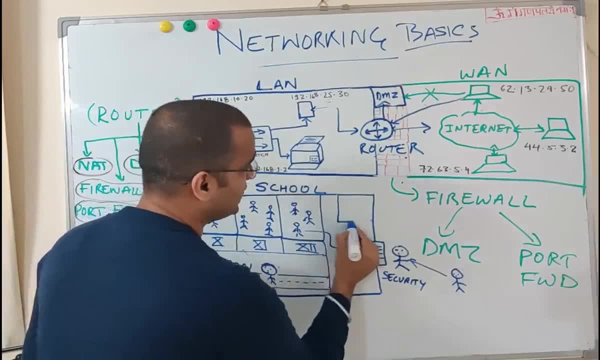 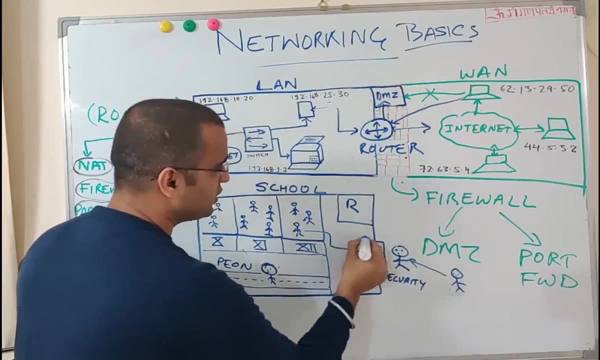 and if there is a dmz setup here it would be actually a kind of a reception here so what security guard can do security guard can simply ask this particular guest to go and wait in this particular reception so that the student can come here and meet the guest or the 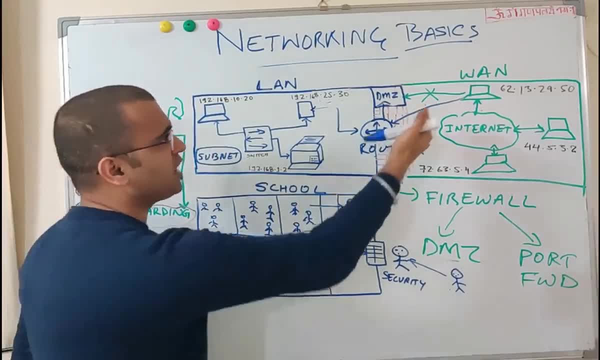 parent port forwarding is another mechanism through which you can you can allow the communication from outside uh network to support a sero on the cloud you want to use code forwarding you want to also sechs other services in the school he will come to this particular security guard 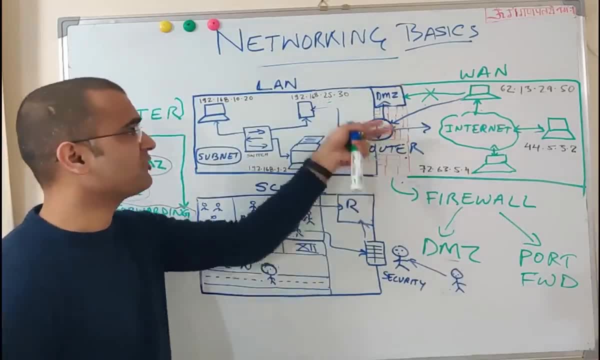 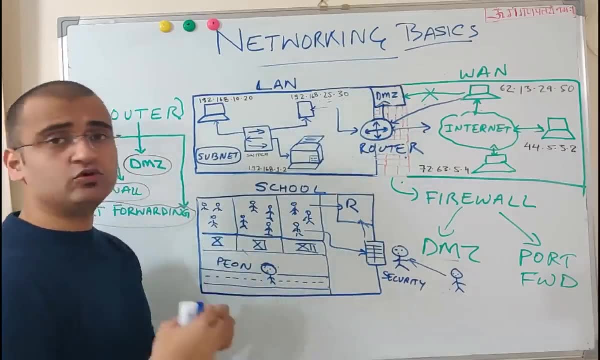 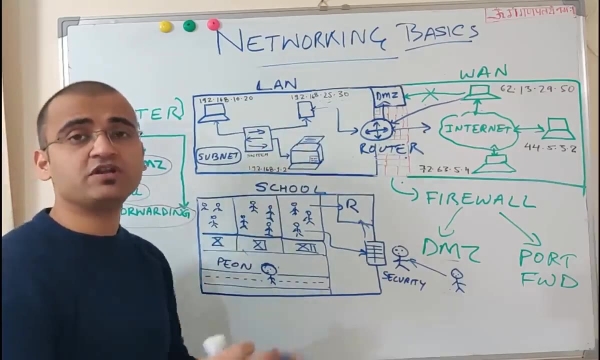 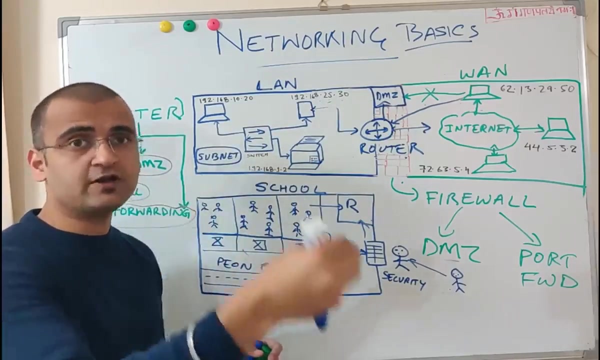 outside network within the local area network through the firewall and the router in the port forwarding concept you do not create a separate dmz rather you specify exactly on which particular port of this particular device or this particular device the communication needs to happen what is a port any machine which is there in the network talks to different machines through different 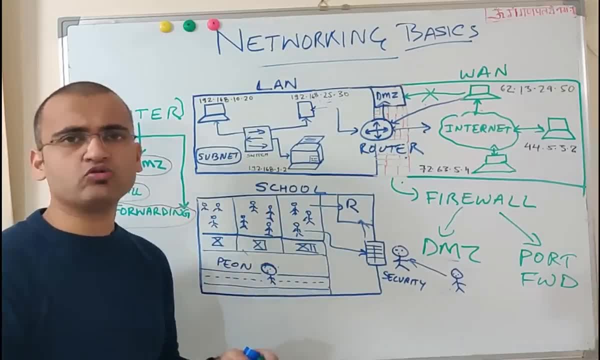 ports so take for example whenever you hit a website on the browser by default it goes to the web server default port which is port 80. you hit a tomcat server it goes to default 8080 if you want to connect to an oracle database the default port is 1521 for every application you need a port 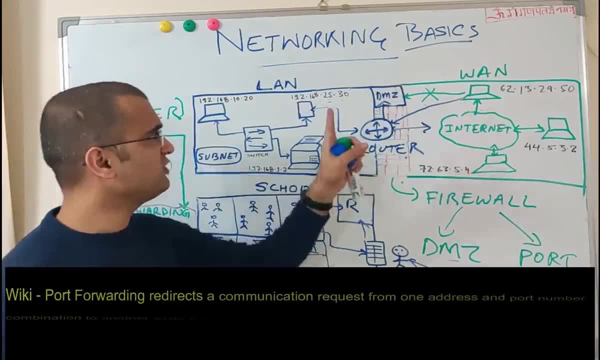 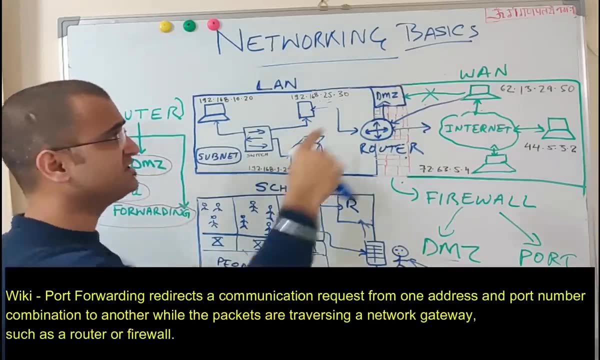 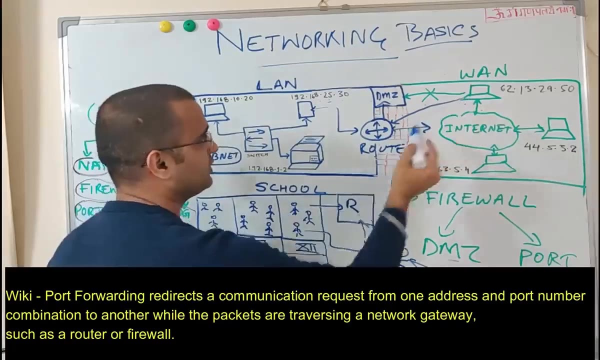 to communicate so suppose this particular device wants to talk to this particular device then in this device there can be a designated port for which this communication can be allowed so . that can go into the firewall rules and it can be written that whenever this particular device 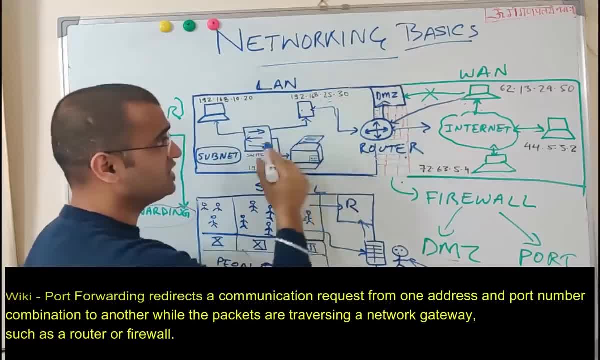 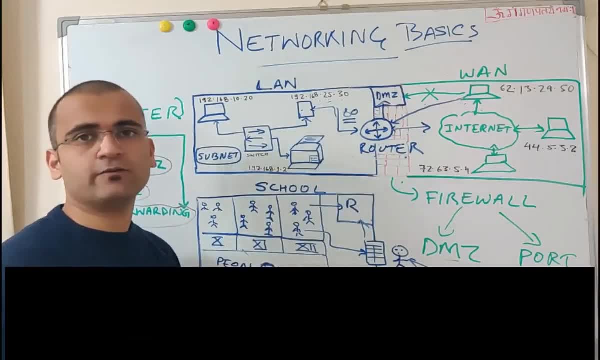 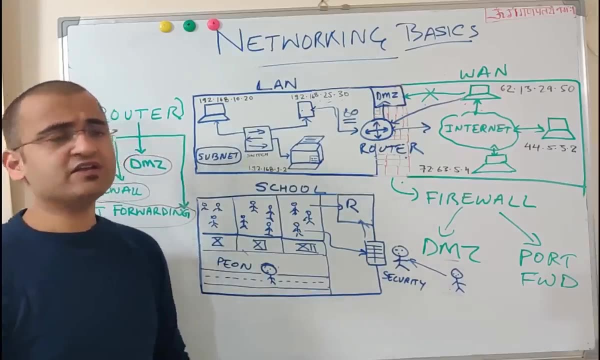 sends a request to this particular device within the local area network on specific port 80 then this particular communication should be allowed without stopping anything so this is the concept of port forwarding so just to summarize we understood the 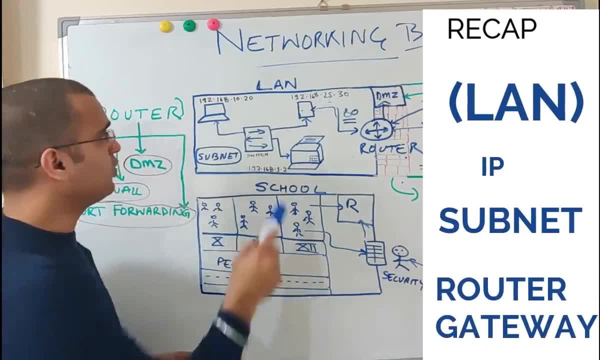 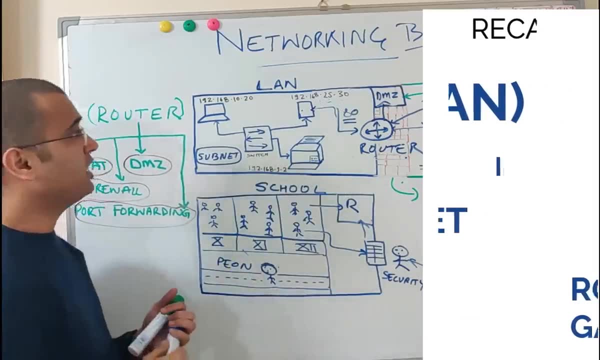 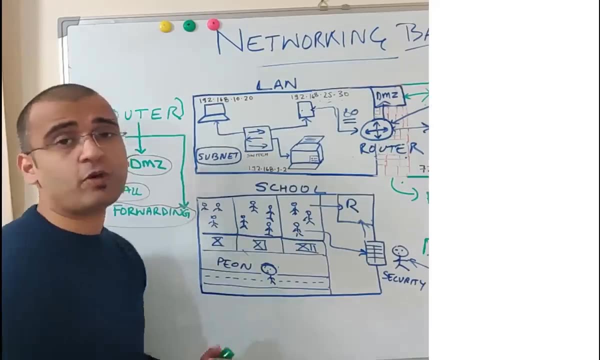 local area network we understood what is an ip what is a switch how these talk to each other then we also understood what is a router what is a gateway we also understand how we use subnet to identify whether a device sits within the network or is actually from outside the network then we moved on to the wider area network we understood how firewall works 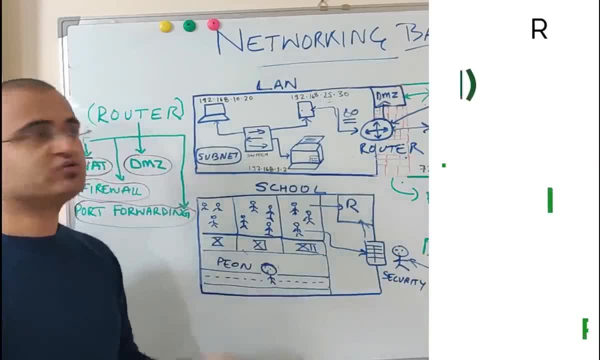 how how dmz and port forwarding are the two mechanisms with which we can allow 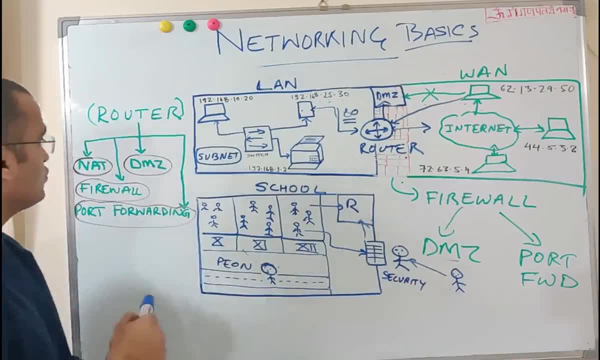 external traffic into the internal network we also understood how network address translation helps 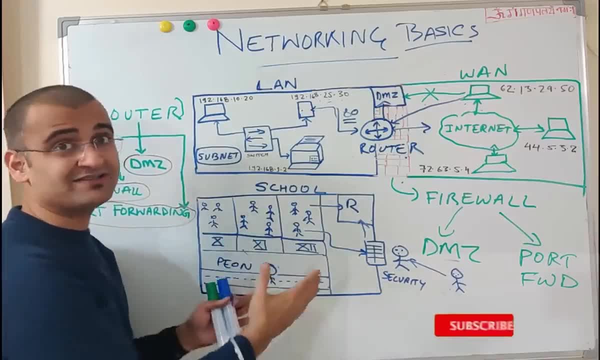 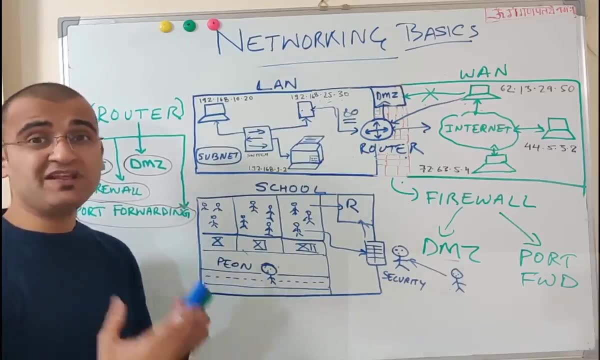 so friends i hope you liked this video and now you understand these concepts in a in a better way please go and subscribe to my channel and hit the bell icon please like and share this video as much as possible and help us grow this community further thank you so much and keep hustling